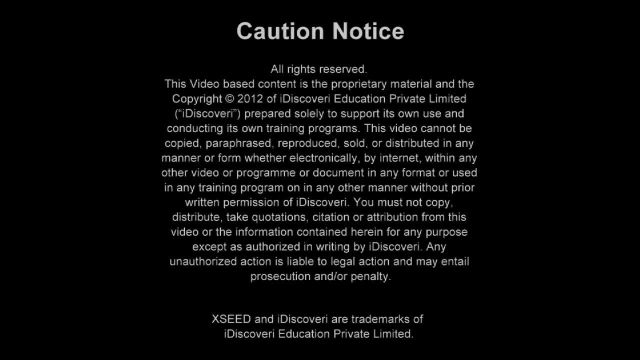 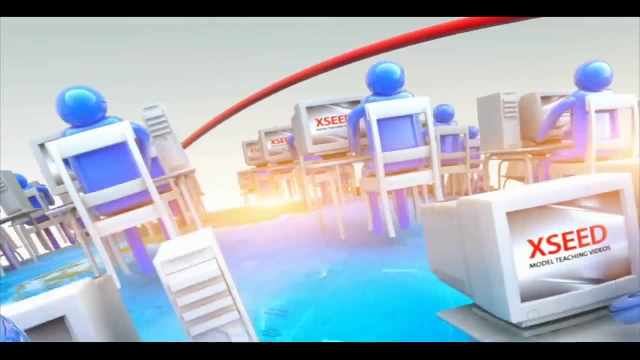 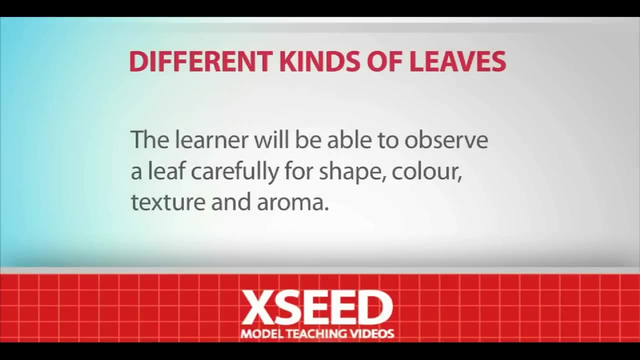 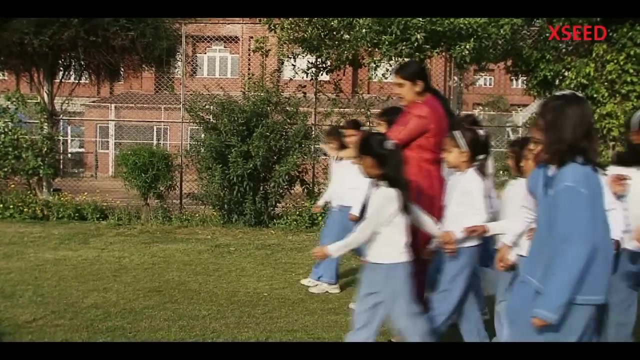 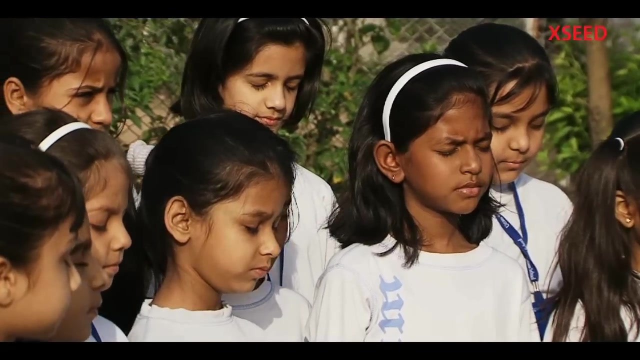 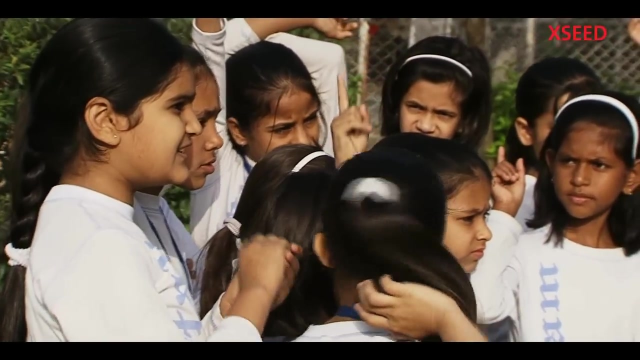 So can we all collect here? stand here. What I want you to do now is close your eyes and see. what are the different colors that you see there: Green, Green. Why do you think that everything looks green? Grass is green and the trees, bushes are green, Leaves are green. 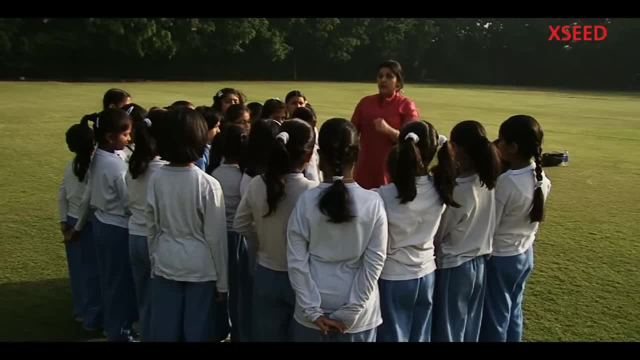 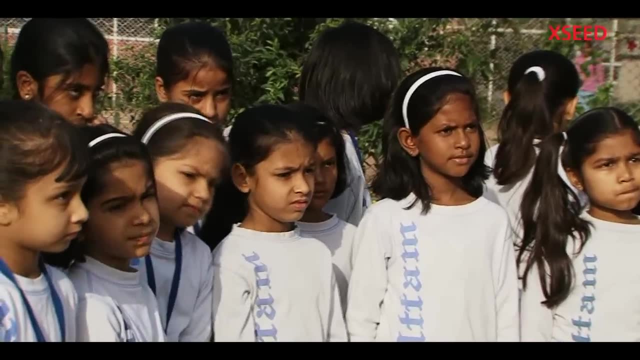 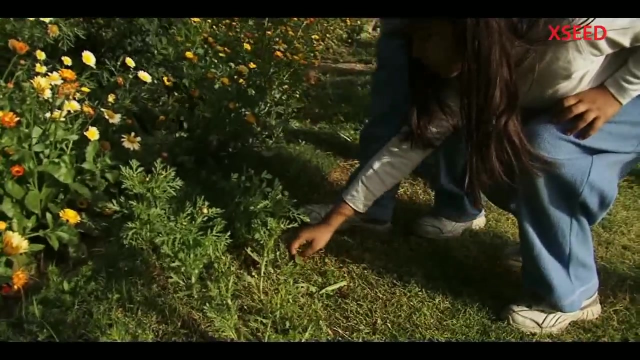 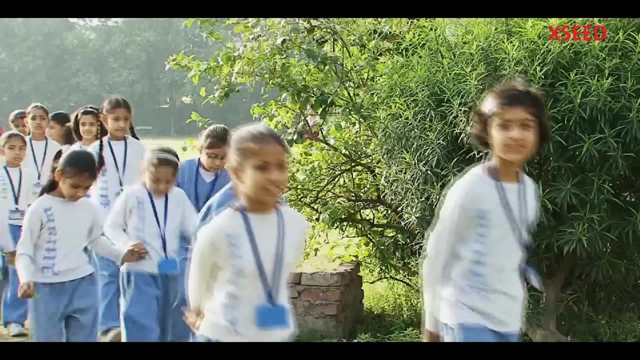 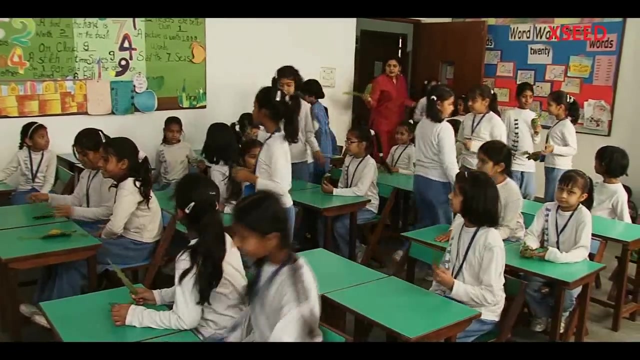 So what I want you to do now is be explorers, nature explorers- All of you will go around, pick, each one of you will pick two leaves of different kinds. So did you have fun collecting leaves? all of you? Yes, ma'am. So how many of you have? 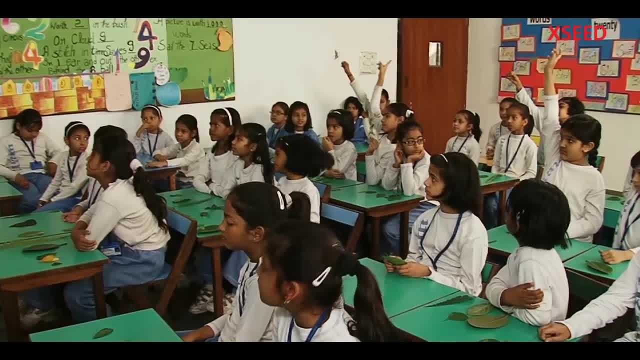 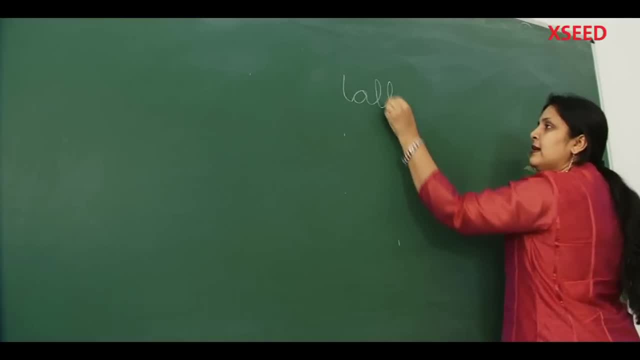 this kind of leaf with you. Just raise your hands. I want you to really look at this leaf and describe the leaf. for me Time, Okay. So what I want you to do now is be explorers, dig Big. So I like the words that you're coming up with. So is there anything else? 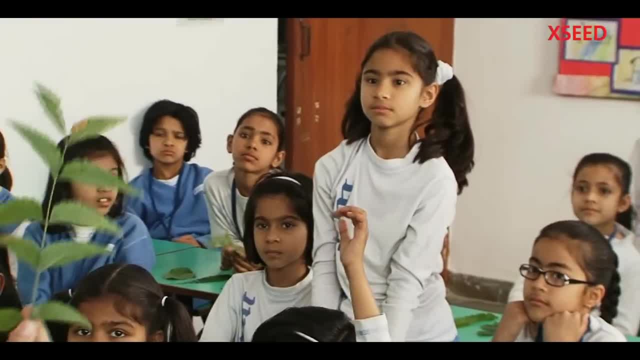 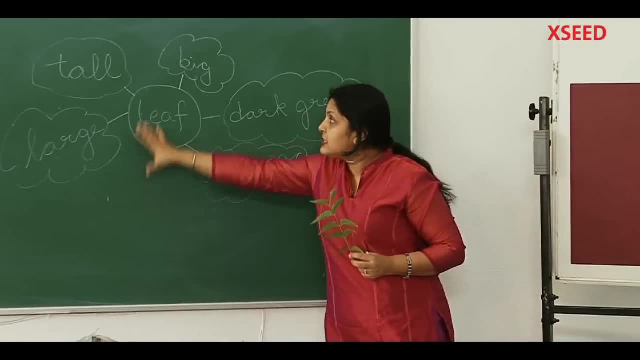 about the leaf. Yes, Ma'am, it's in dark color. It is dark color. Which dark color is it Dark green? It's laser zigzag. Some of you said that it is large. some of you said it's tall. some of you said it's big. What else? Huge? Oh, that's another word which she's saying. 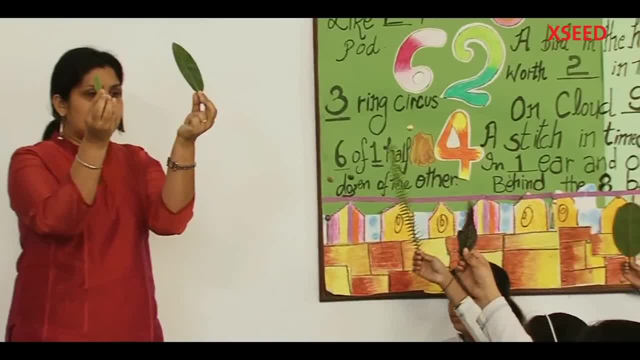 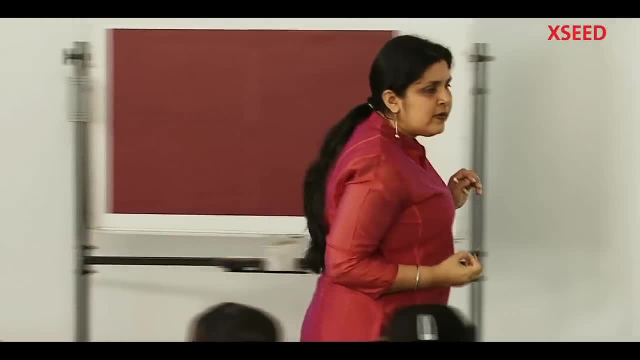 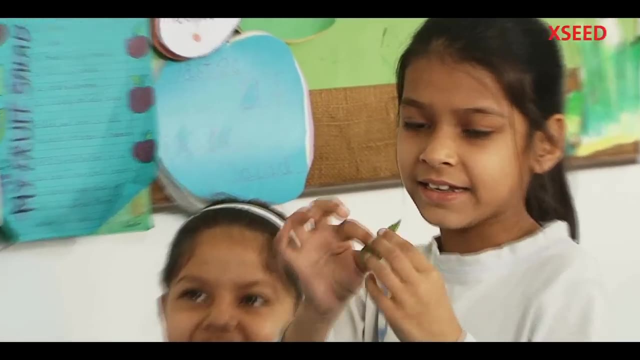 huge. This one is comparatively huge, So this is huge. So what will this be? Small, Small, Small. Anything else about the leaf? Yes, Ma'am, it has two colors. Can you show us how, Ma'am? this one is light green and this one is dark green. Lovely, That's. 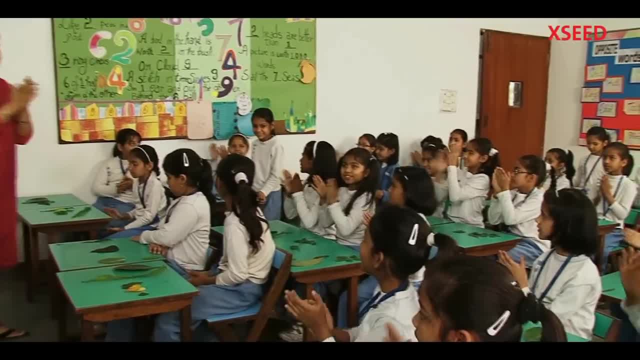 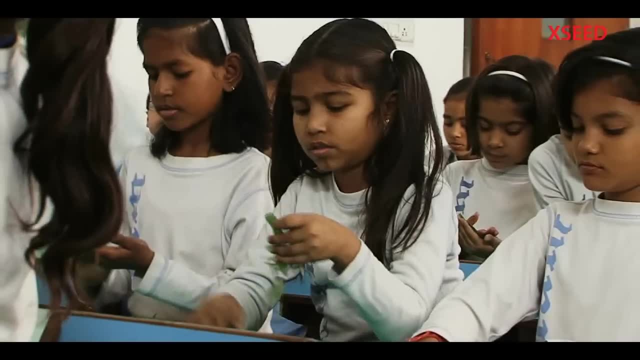 a very good observation. Can we clap for her? Can you quickly feel the leaf and tell me It is soft? So all of you touch all your leaves and see what are the different kinds of textures. It is hard, It is hard. Okay, Let's see. 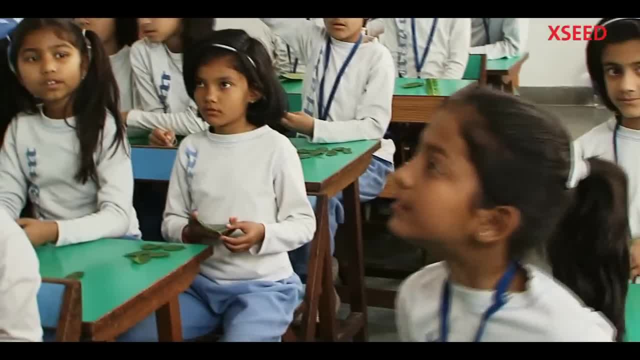 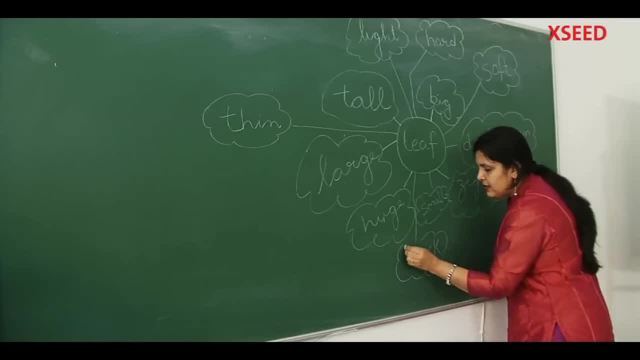 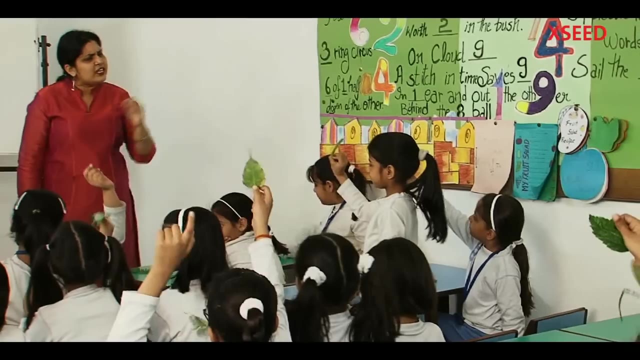 Let's put that up. It's very thin, Thick, Thick. So some of your leaves are thin while some of your leaves are thick. Is there any other kind of? They are very smooth. Smooth- That's a nice word, Ma'am. it is dry. Why do you think it is dry, Ma'am? I'm touching it. 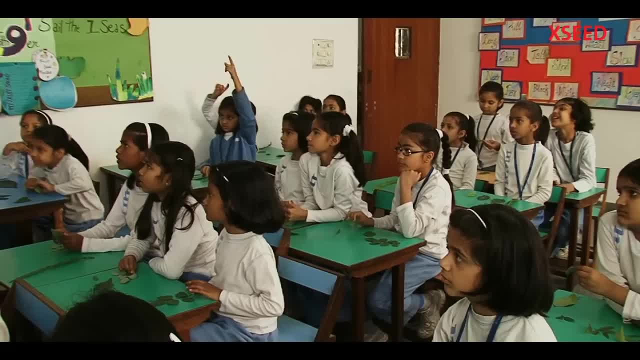 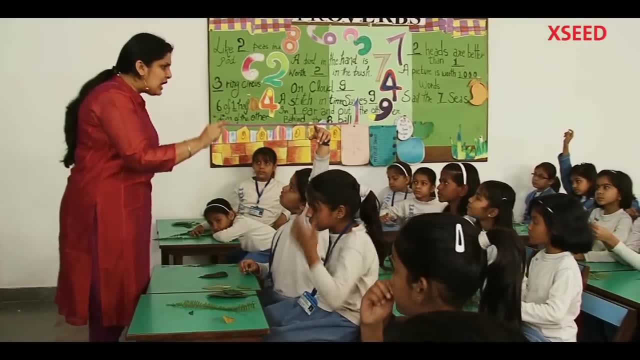 Is this leaf dry? No, Some parts of this leaf dry, Yes. Do you know what is margin? Yes, Ma'am, it's the margin. You know that the outer part of a leaf is called margin. Is that clear? Now I want you. 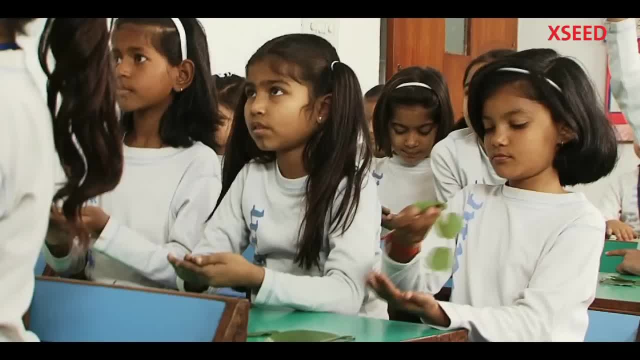 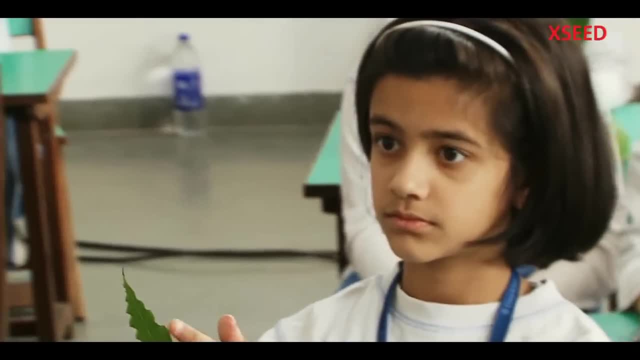 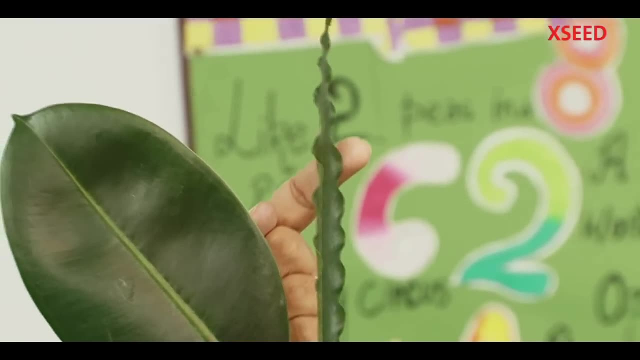 to look at your leaves and find out what kind of margins are there on your leaves: Curve, Curve? Okay, Is this curve? No, Oh, so you say that is curve. So there are curves on this. See, from the bottom of the leaf to the tip of the leaf there are curves, Small curves. 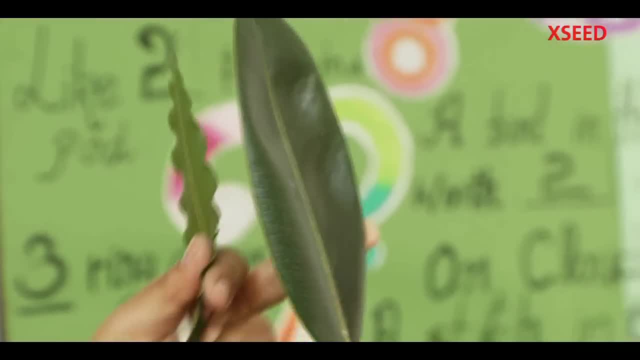 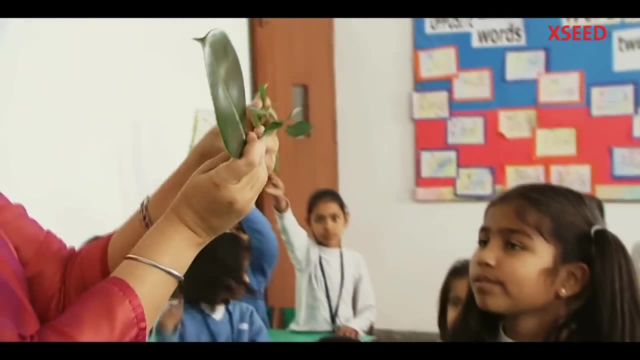 on the leaf, So this one doesn't have curve. What kind of margin is this? Narrow, Narrow, So this is a sharp margin, Very nice. So I want all of you to look at the rose leaves and see if you touch them, you will see that they can a little. they. 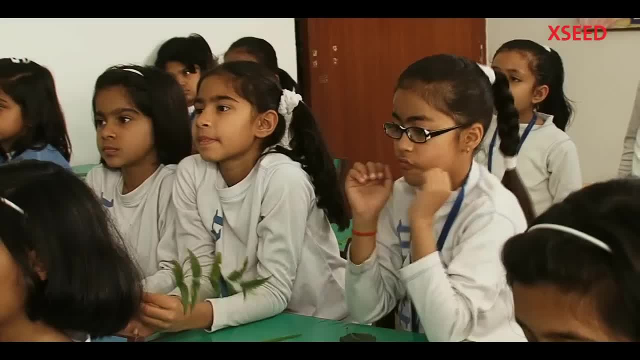 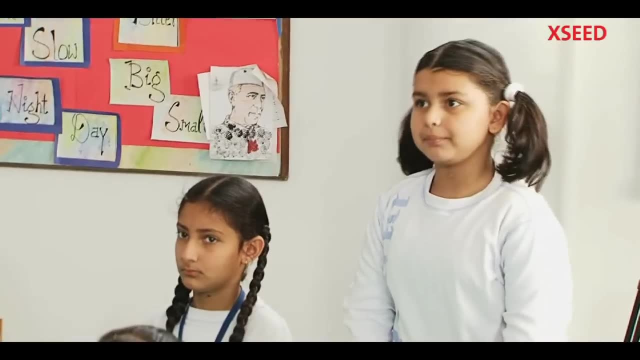 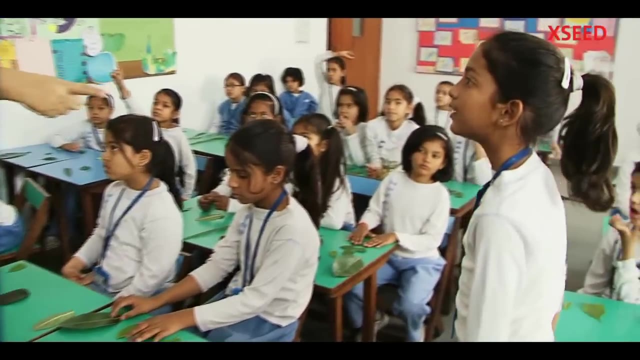 can prick you a little, So they are sharp margins. What are the different things up till now that we have described about the leaf? Colour, Sizes, Margin, Shape Material. What is that? smooth or Material That's very good. Can we clap for her? 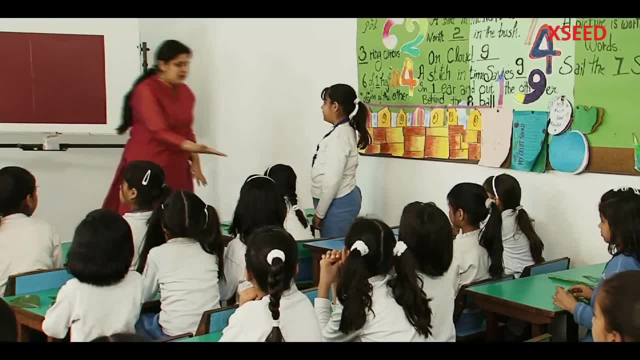 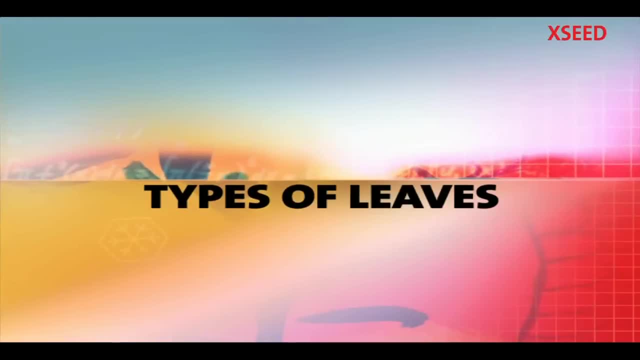 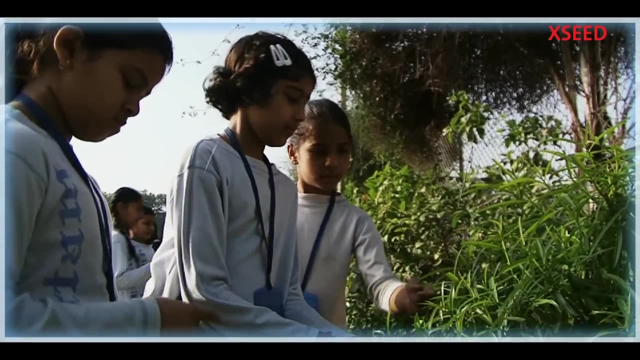 Some other words for material Texture. Texture Gimme a high-five Haan. Did you know that we can describe a leaf in so many ways? No, Trees & plants have leaves which come in many different shapes, sizes and colours. Some. 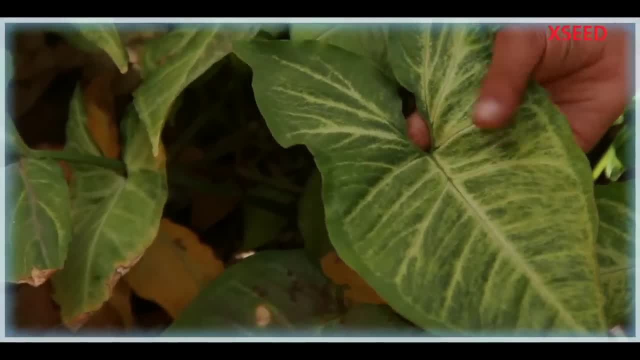 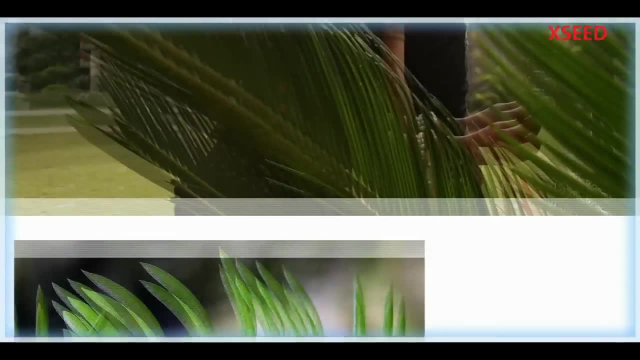 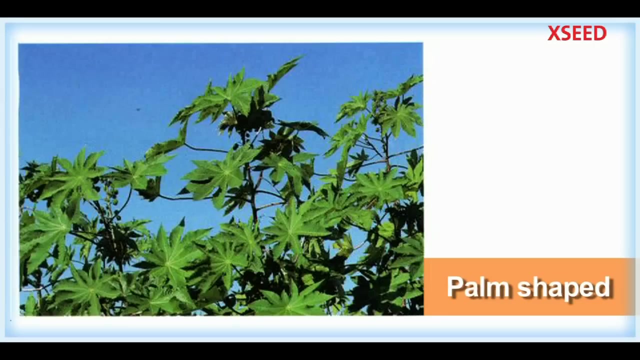 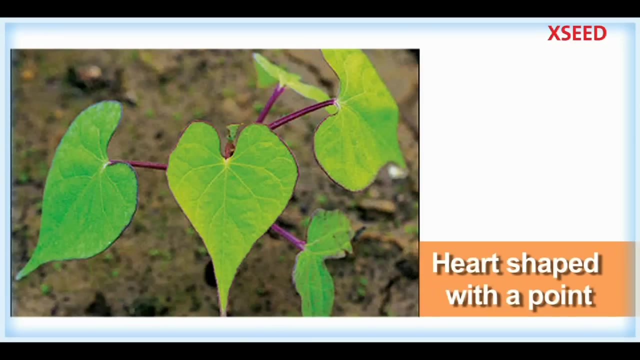 are needle shaped, while others round, Wow, Wow- can be heart shaped, oval or even circular. they also have different patterns on their edges. leaves can be sickle shaped, needle shaped, circular, diamond shaped oval, palm shaped, heart shaped, leaflet shaped or heart shaped with a point. leaves can have different textures too. 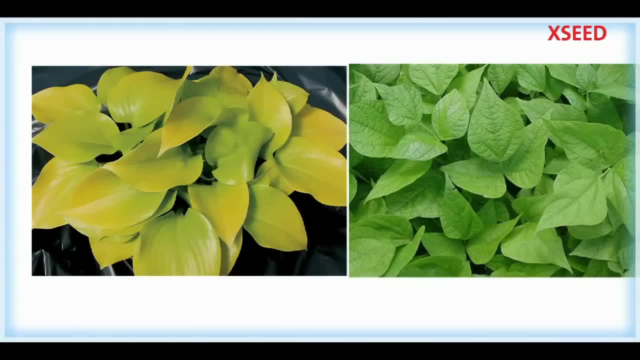 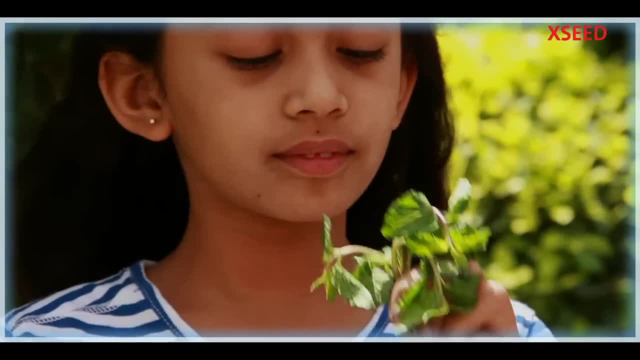 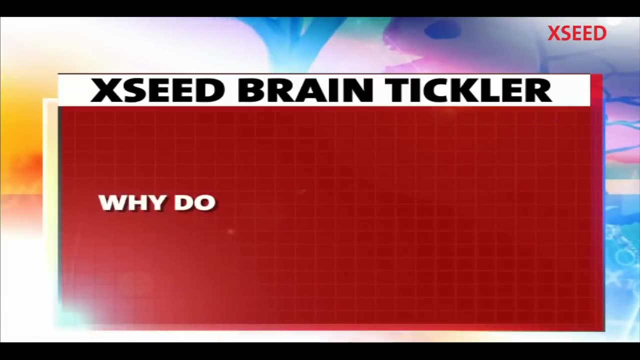 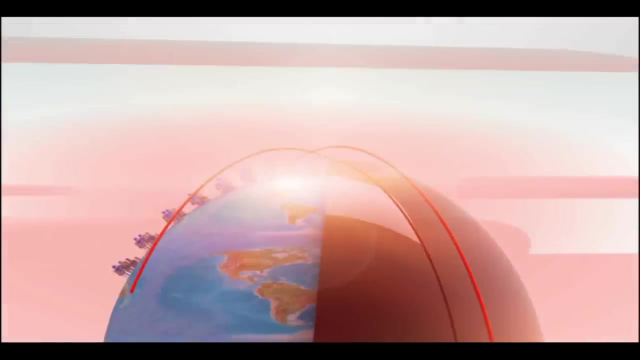 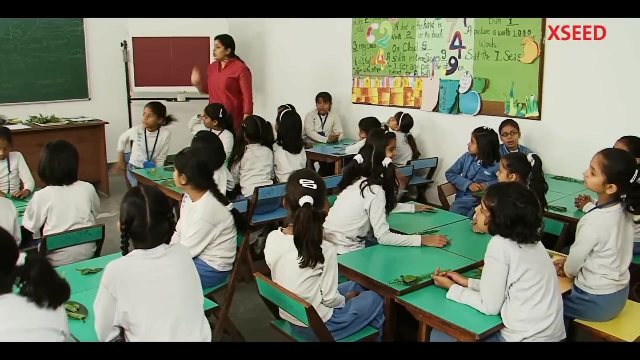 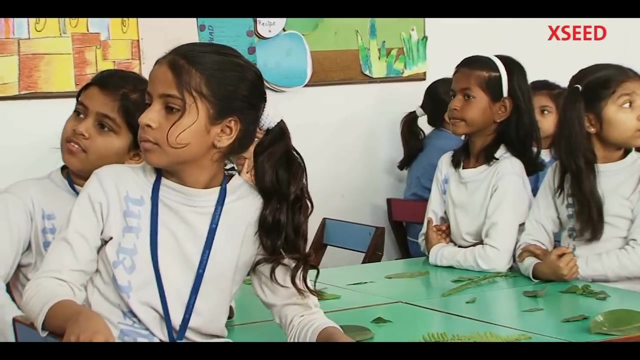 some are smooth, while others are rough. they may have different shades of green and may even be differently colored. some leaves can be identified by their special aroma or smell like mint leaves. why do plants have different kinds of leaves? so, since we have so many words on the board and so many different ways to describe a leaf, what we are going to do is 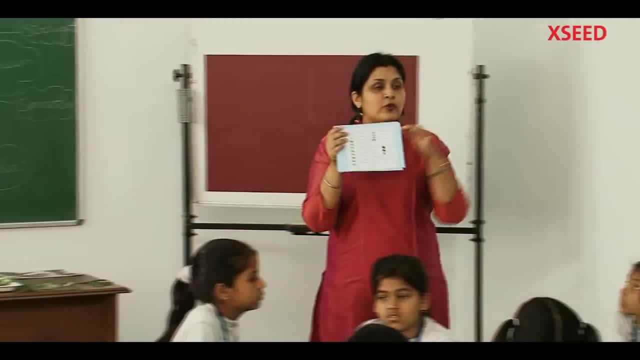 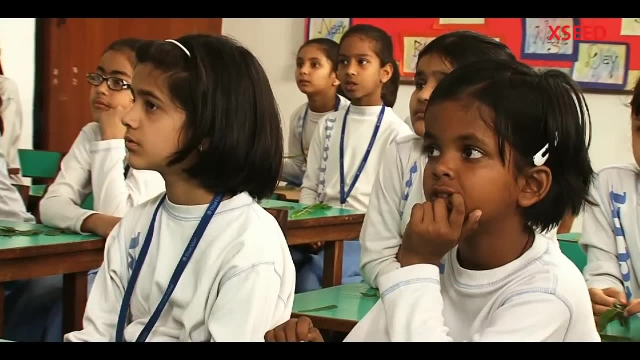 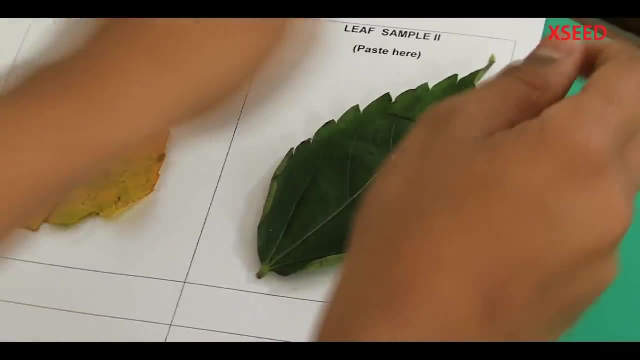 we are going to choose some words each group. i am going to give you a card like this. you have to pick two leaves of different kind. after pasting the leaf, you have to observe. look at the leaf, see in your card to describe what type of leaf looks like this: 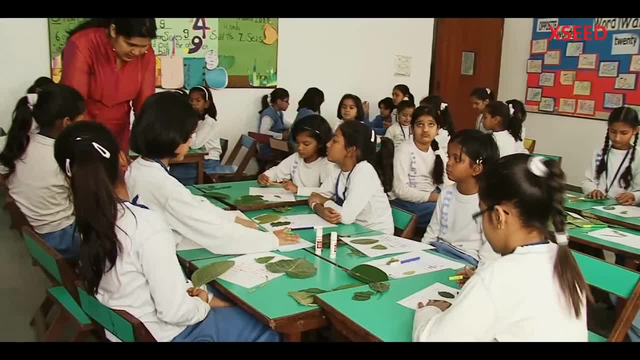 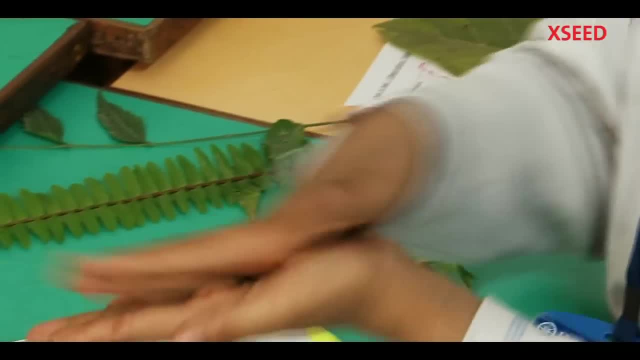 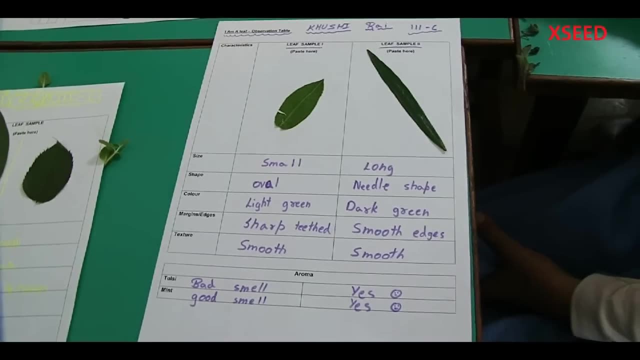 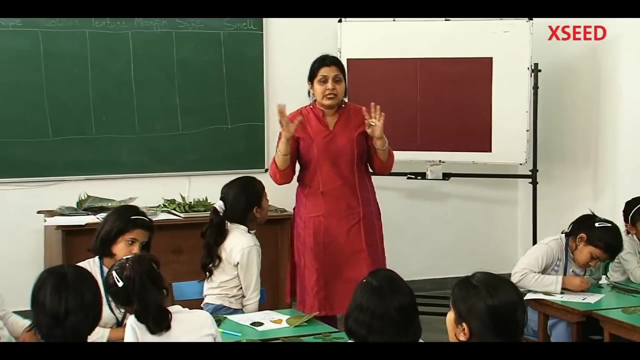 so i'm going to give you another kind of leaf, rub it on your palm and then smell it and tell me whether it has smell or no. Can anybody tell me what are the different kinds of ways you have described the leaf? Oval Oval Heart. 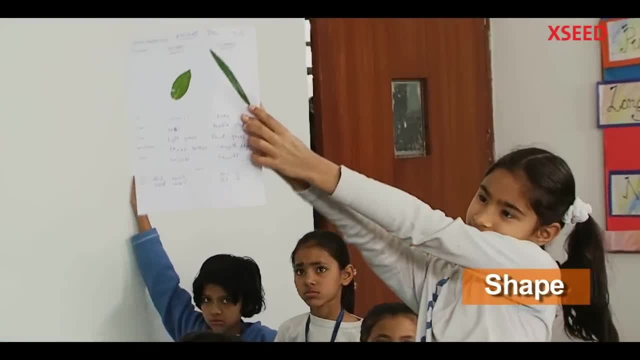 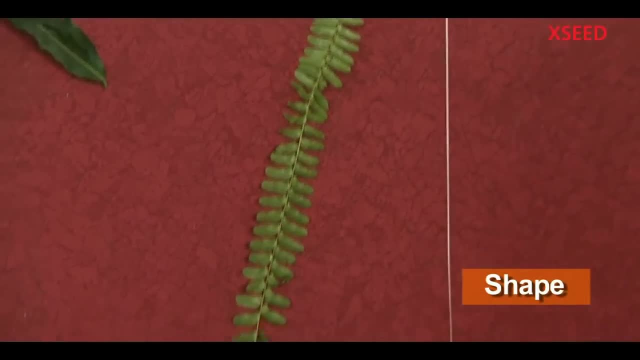 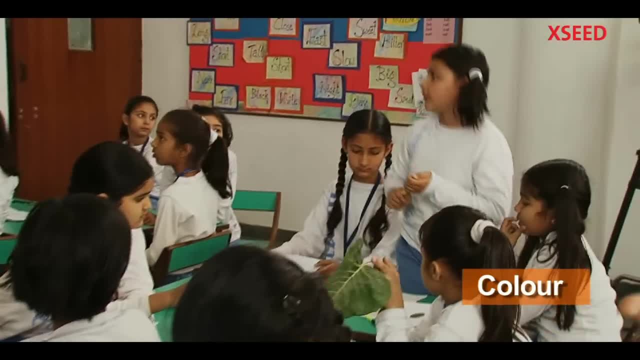 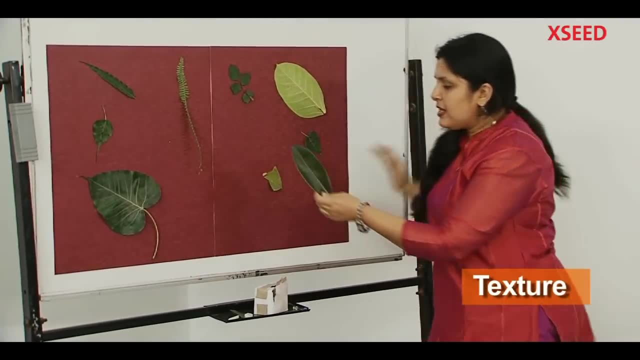 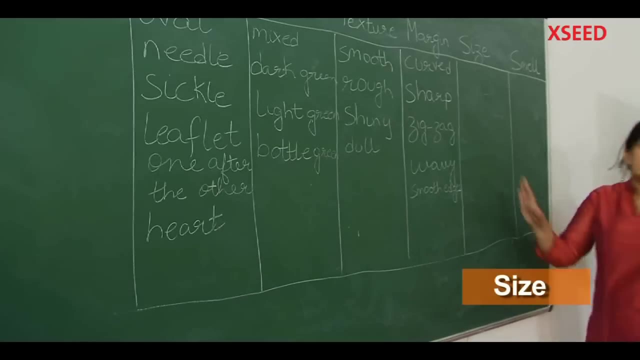 The light green, Bottle green, Bottle green. Smooth, Shiny, Rough. So this is the rough one and this one is smooth, Curve, Curves, Curve, Sharp teeth, Curve baby. Let's come to size now: Dirty. 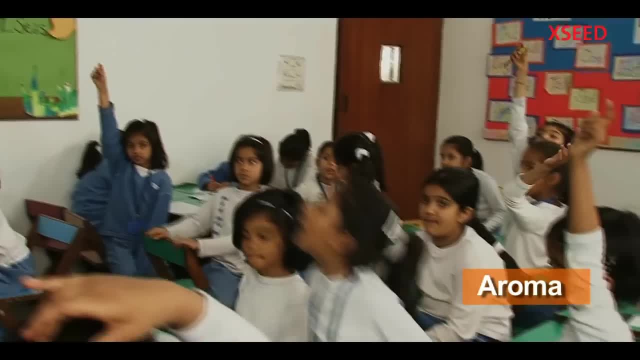 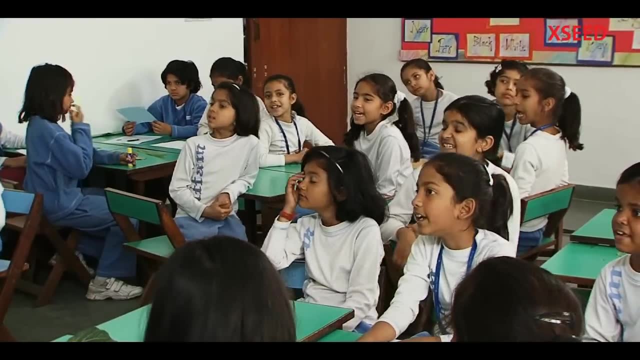 Big, Big, Hard, Good smell, Unusual smell. Wow, That was very interesting. Was it interesting for you? Yes, What was interesting? More the trees, more the leaves. Now, this is a group activity. Alright, I am going to give you this sheet. 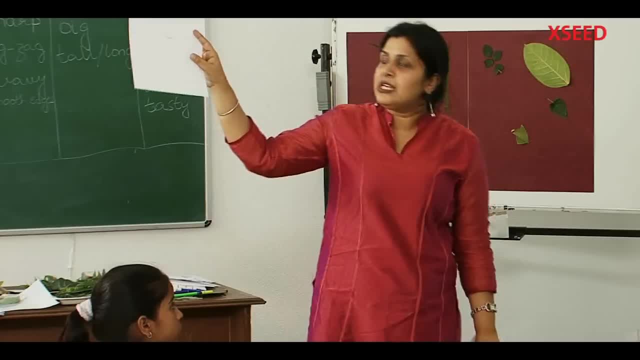 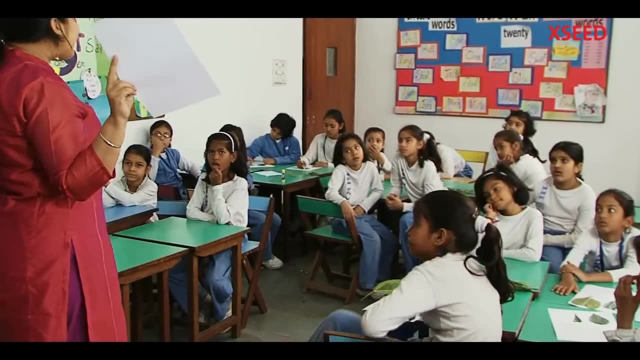 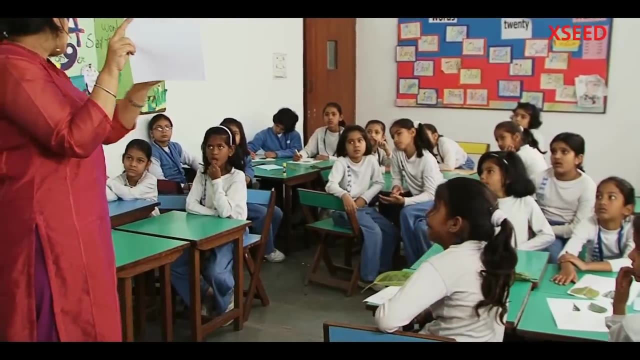 This sheet has four boxes and I am going to also give you pictures And I am going to read something for you. You have to look at the picture and decide which picture will go in which box. I would live in house number one. I am dark green in colour. 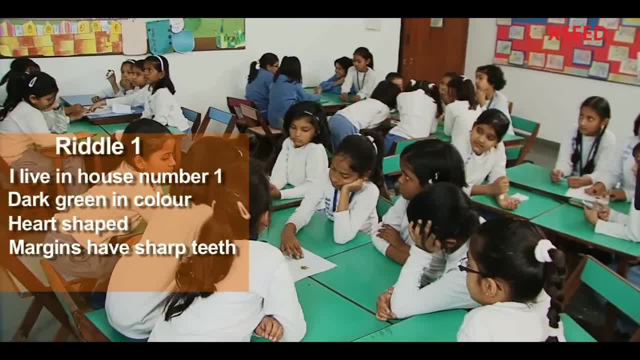 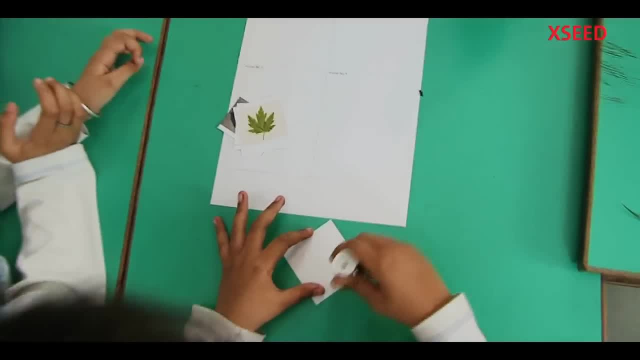 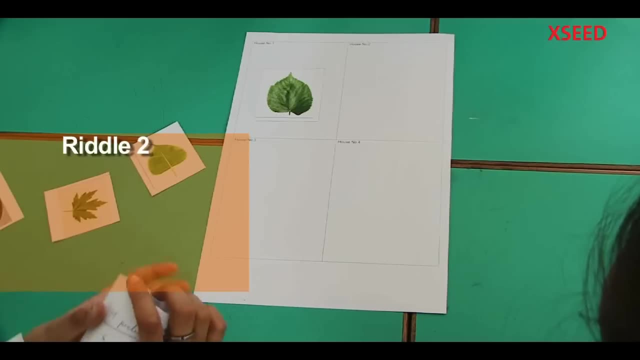 I have a heart shape. Touch my margin carefully, as they are sharp teeth. Who am? I Choose it for house number one and paste it. Can I read the second one now? Yes, ma'am, I would live in house number two. I am bottle green in colour. 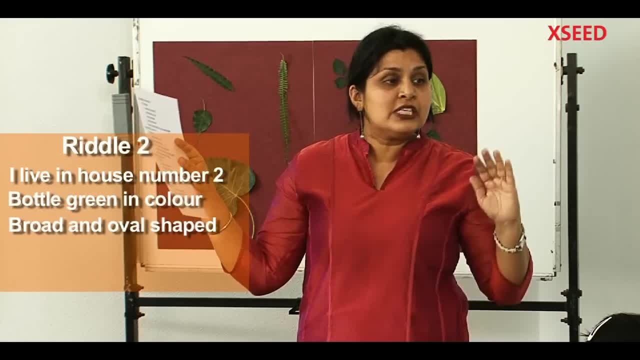 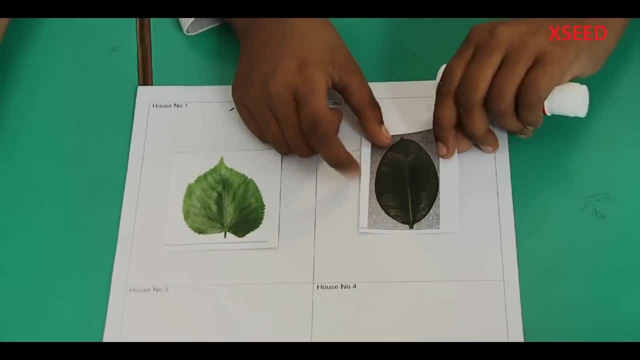 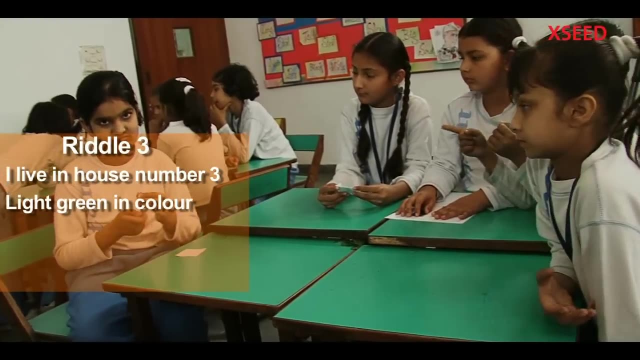 I have broad and oval shaped leaves, But my edges are round. My edges are plain. Who am I? Can we move on to the third one? I would live in house number three. I am light green in colour. I also have a heart shape. 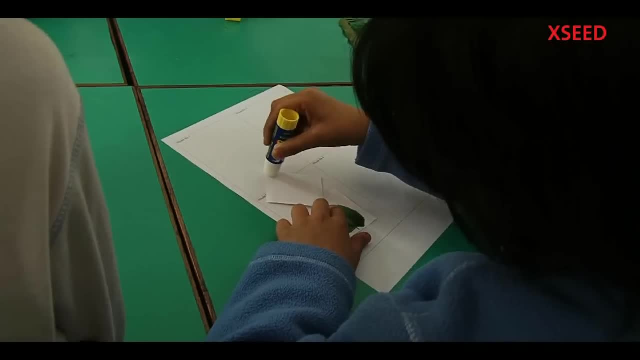 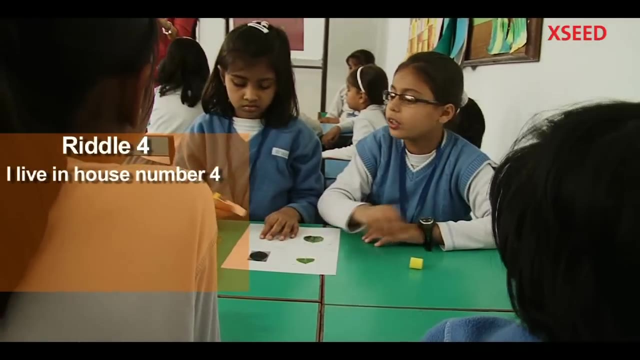 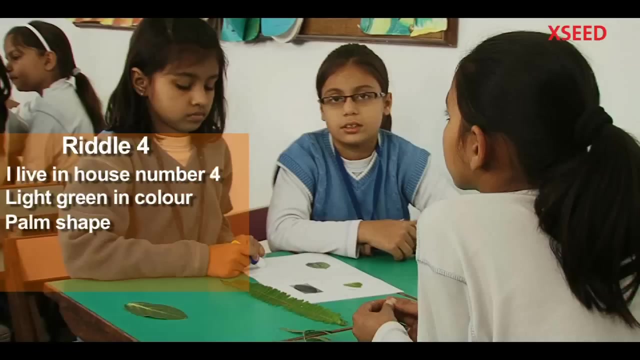 But my tip is a bit longer. Who am I? Now, let's do the last one. I would live in house number four. I am light green in colour. I have the same shape as your palm. My edges are toothed. Who am I? 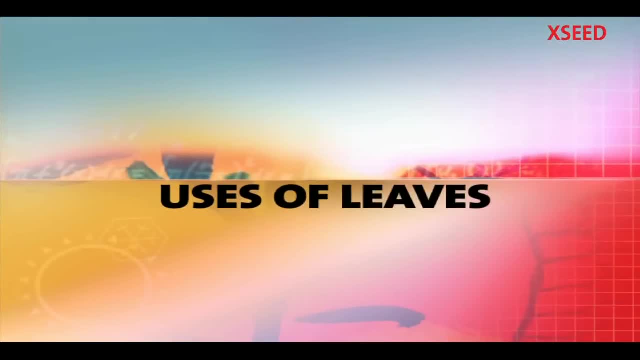 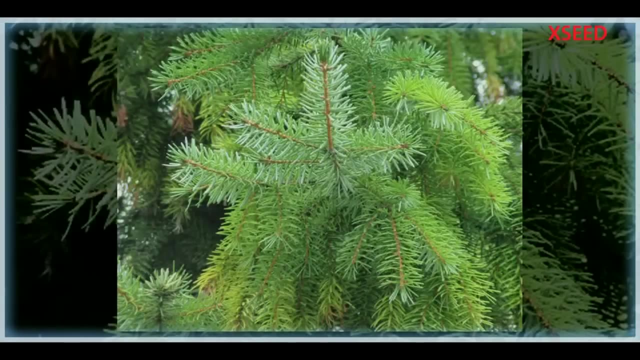 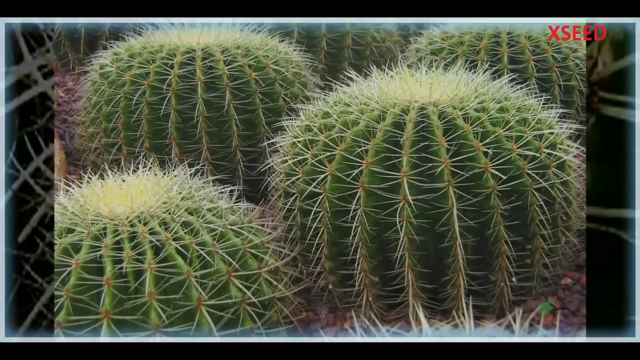 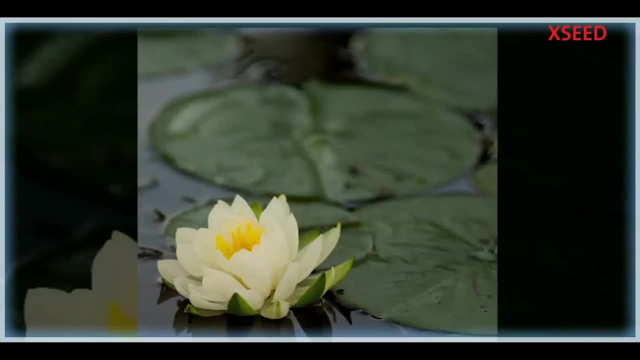 Done. Interestingly, the different shapes, colours, textures and margins of leaves help the plant or the tree to survive in their surroundings. The large leaves of the lotus are broad to enable the plant to float in water. Some leaves have shiny surfaces to minimize water loss. 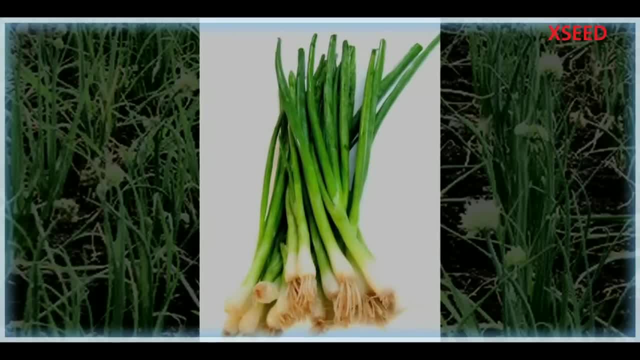 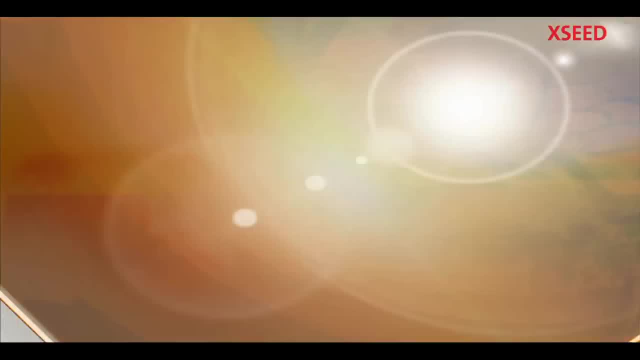 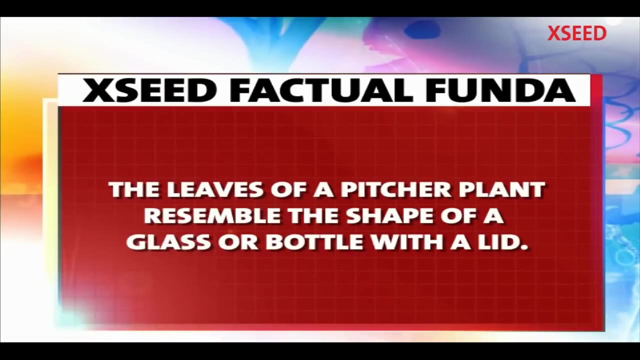 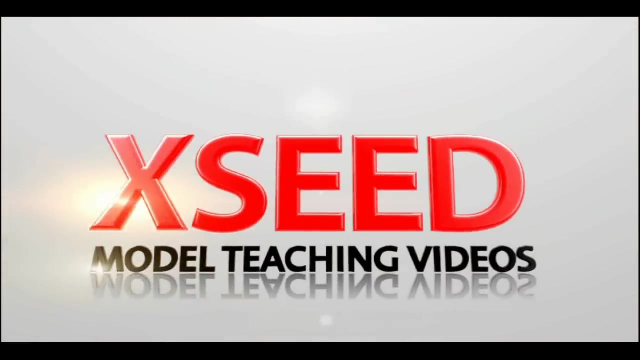 Some can store food and water like onions, while some are large to get more sunlight to the plant. The leaves of a pitcher plant resemble the shape of a glass or bottle with a lid. Now that we know that there are different kinds of leaves, do you think the difference? 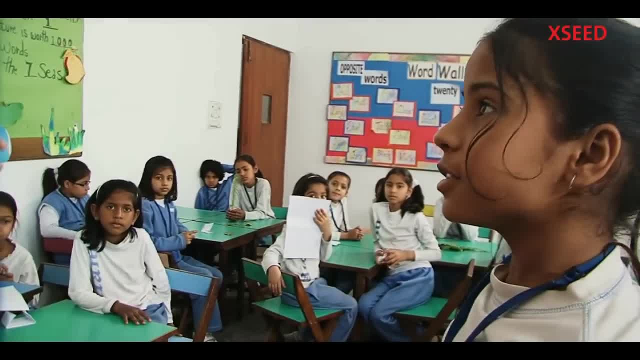 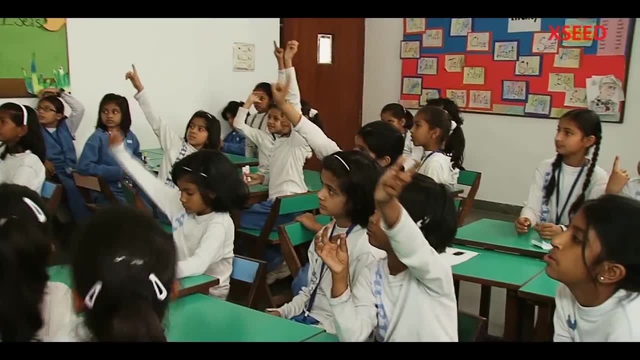 in the leaves helps the plant in any way, Make it beautiful. It makes it look beautiful. Okay, have you all seen a cactus plant? Yes, I have seen it. So here is a cactus plant. Do you think that the cactus plant has leaves? 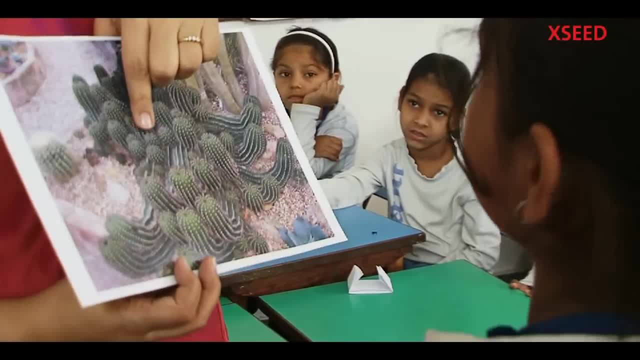 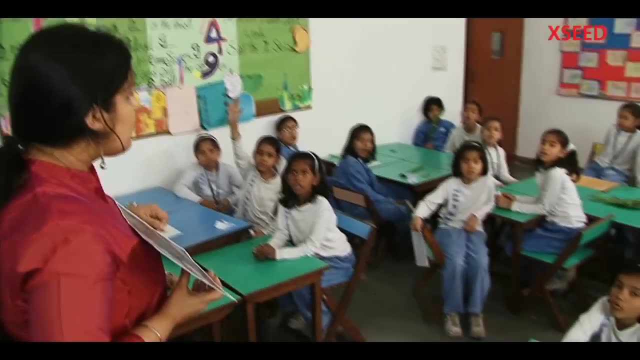 Yes, it has white leaves. This white white thing are the leaves of cactus plant. So what kind of leaves are they? Small, Small leaves. Why do you think that the leaves are small? Okay, tell me. have you seen a tap in the washroom? 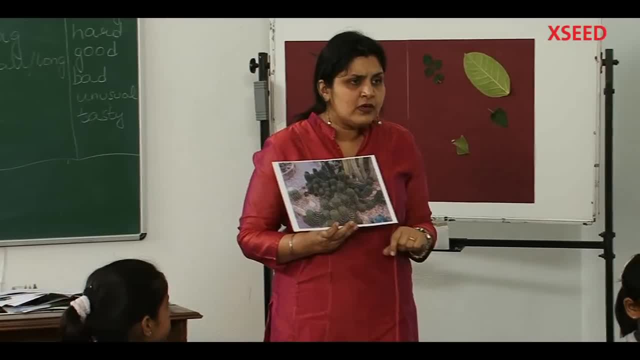 Yes, How much water does come out from a tap? Lots of water, Lots of water. Have you seen a shower in the washroom? Yes, So how much water comes from each hole? Lots of water, Little bit, Little bit. 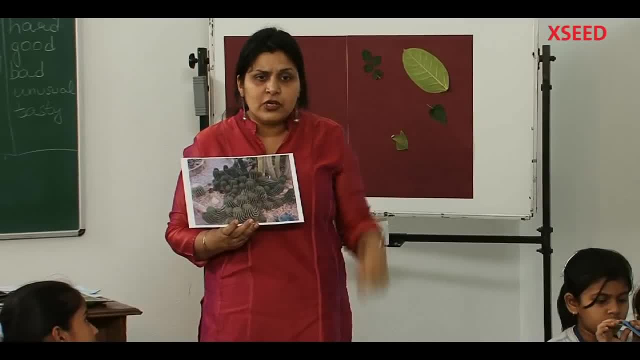 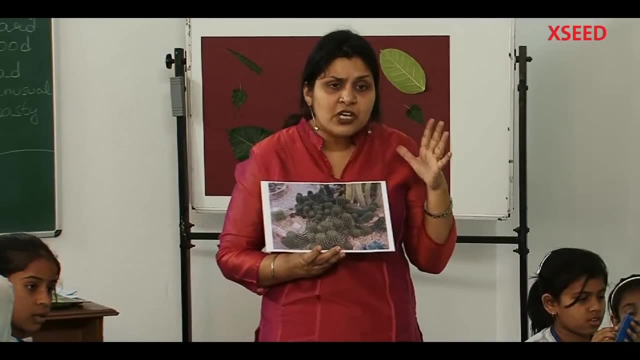 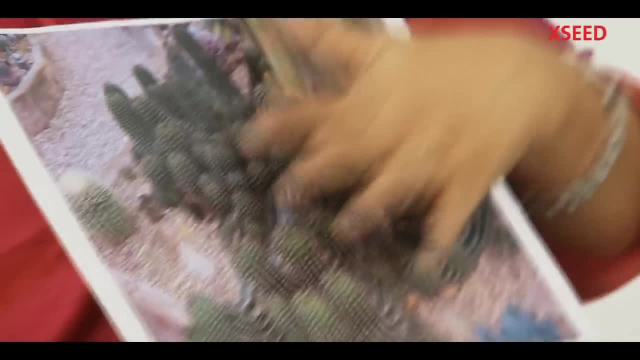 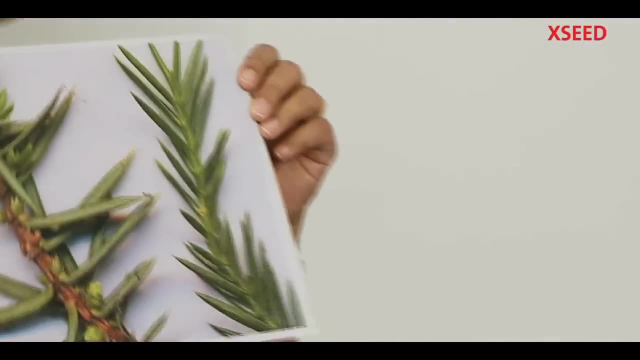 Little Little. This quality of the plant, of the leaf, helps the plant to live in a desert. So lets look at a picture. These are found in places where there is lots of snowfall. How do you think this kind of leaf shape helps the plant? 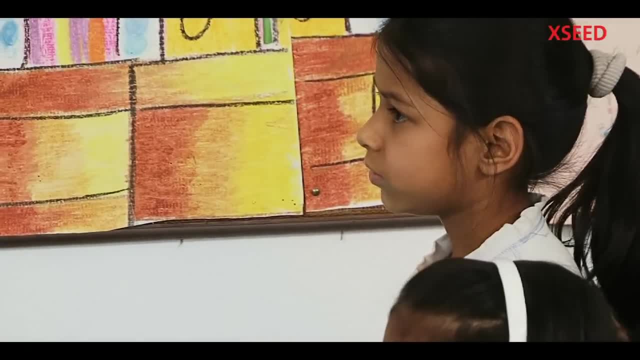 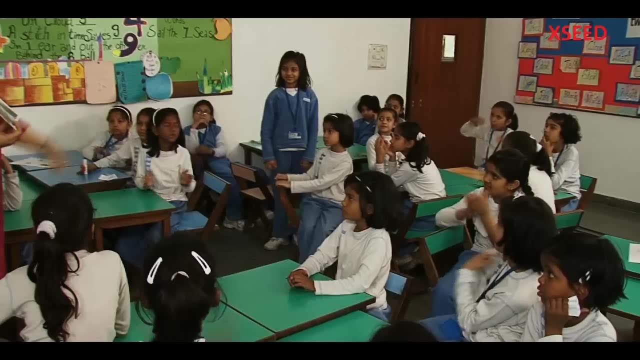 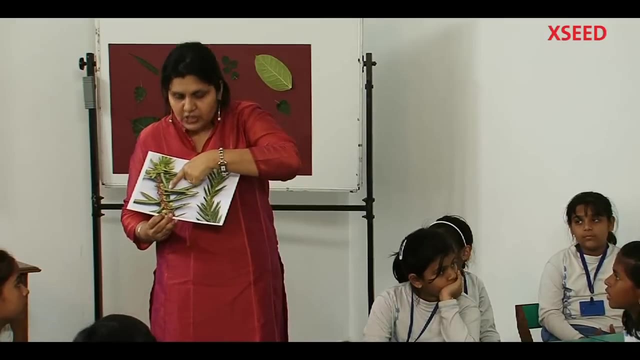 Protecting them from snow. How do they protect them from snow? The snow, the pebbles, snow slab down from this triangle. Excellent, Can we again clap for her? The snow that falls on this tree, it melts and it falls down, So the roof is like this in the 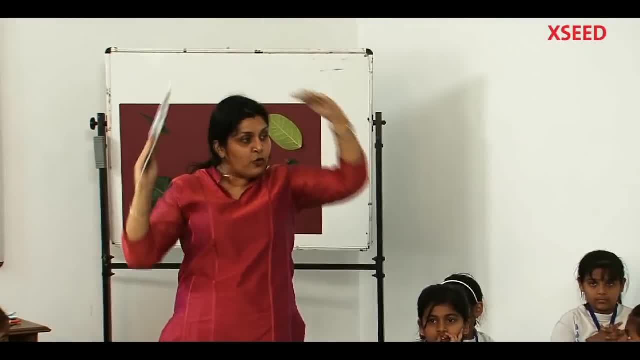 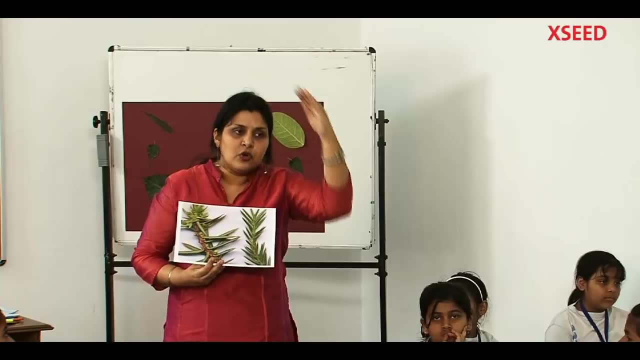 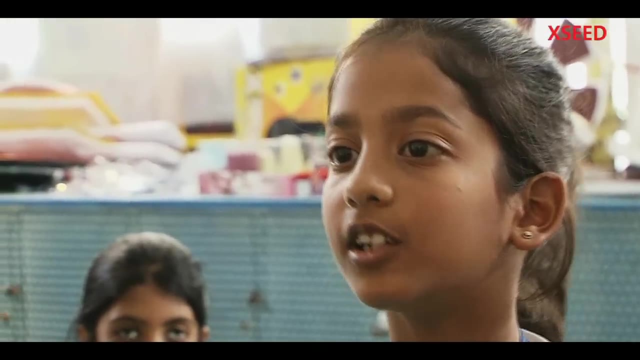 areas where there is snowfall. Yes, So even the roof helps for the snow to fall and doesn't collect on the rooftop. Similarly, this kind of leaves help the snow to fall and not collect on the leaves. What do you learn from these examples that I gave you, Ma'am? we have learned that all. 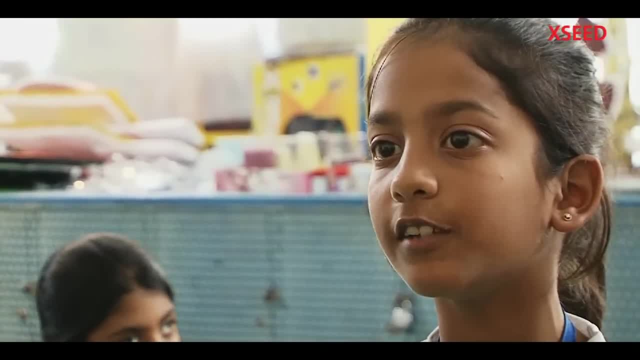 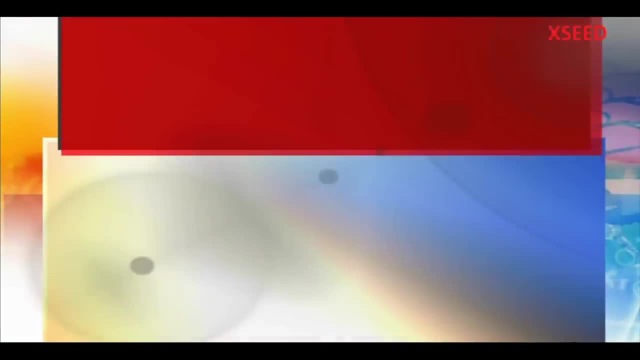 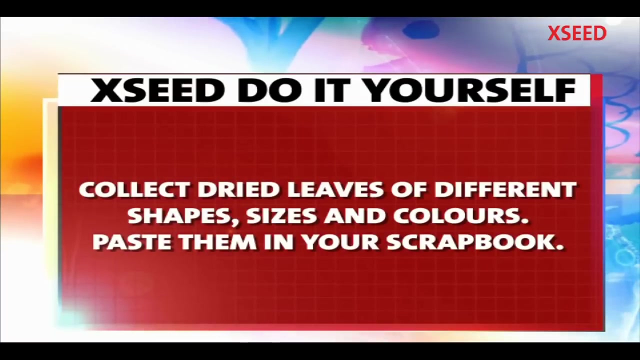 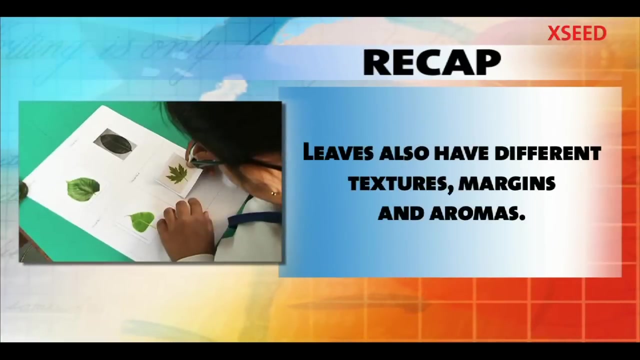 the qualities of these leaves help the plants to live in that particular place- Excellent. Can we all give her a nice clap? Yes, ma'am, we have learned that all the qualities of these leaves help the plants to live in that particular place- Excellent.